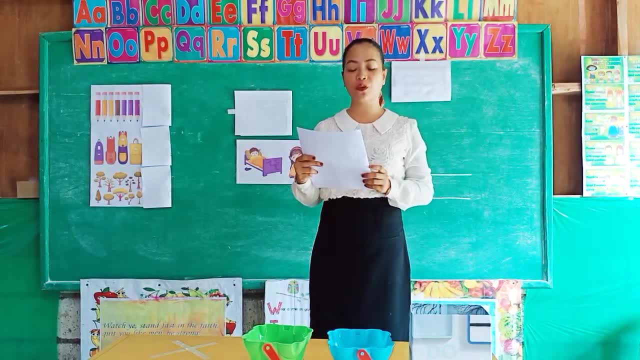 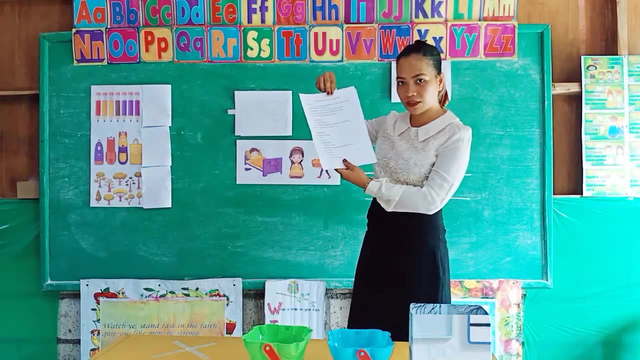 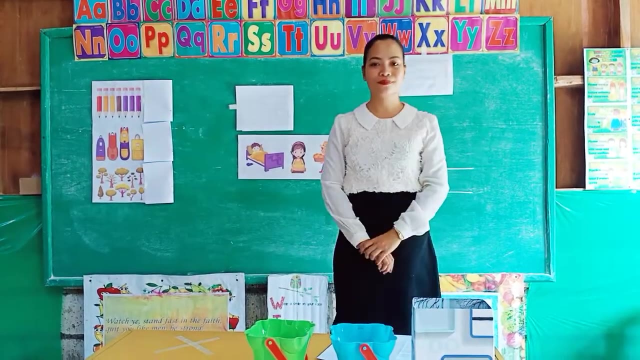 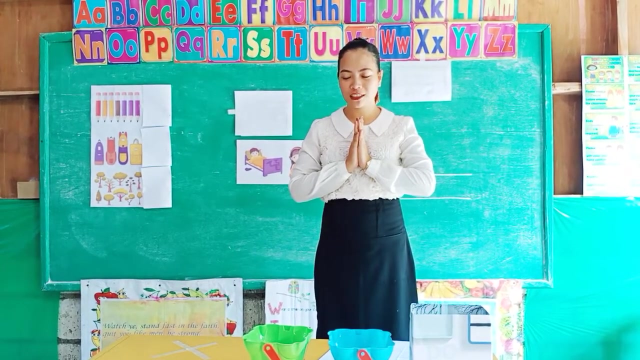 They will also add and write addition sentence for a given set of objects. They will count and add diligently the objects or the numerals. So I will start Grade 1,. please stand up. We will pray. Follow teacher. Dear God, we thank you for this day. 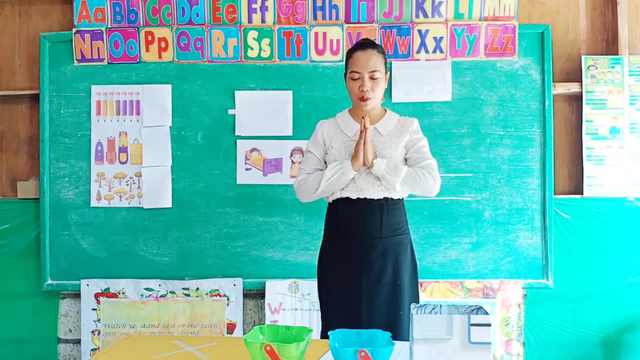 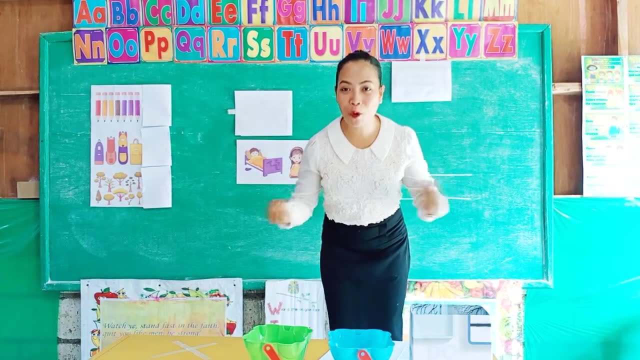 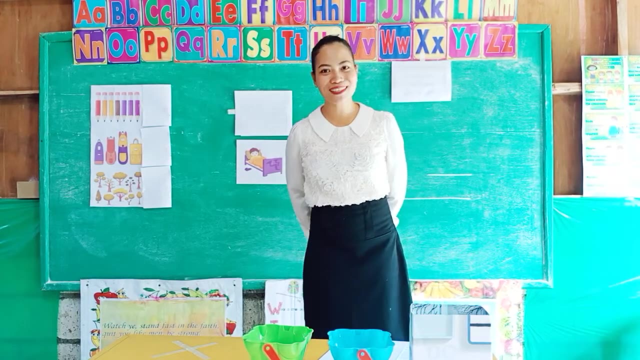 We are asking for your help as we have our class This all. we pray in Jesus name, Amen. Good morning grade 1.. Good morning kids. Hello, How are you today? Good to hear. So are you still absent from class in grade 1?? 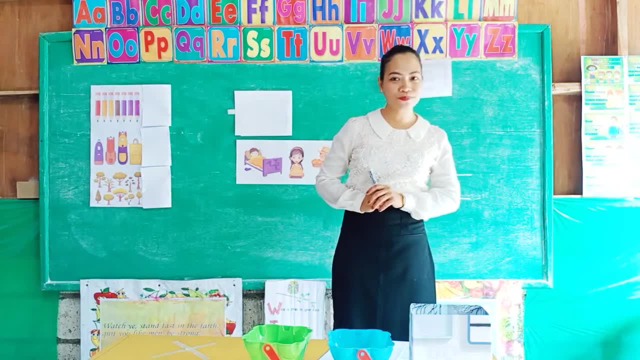 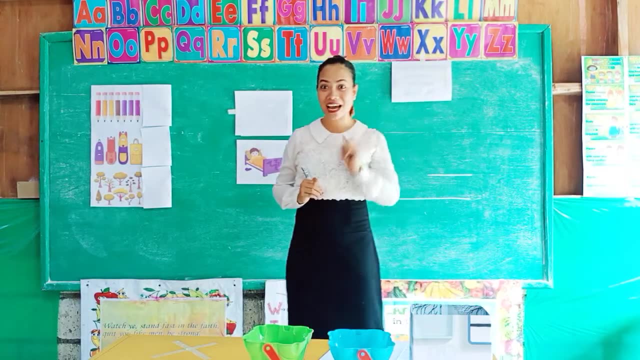 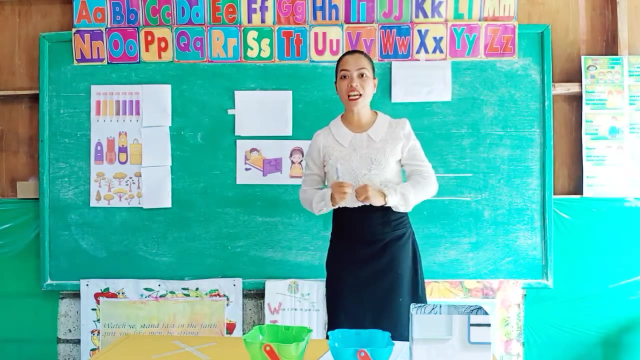 Look at the boys. No, Very good, No one is absent. How about the girls? Okay, No one is absent. Very good, Clap your hands. So now we will have our new lesson, But before that we will review what we had yesterday. 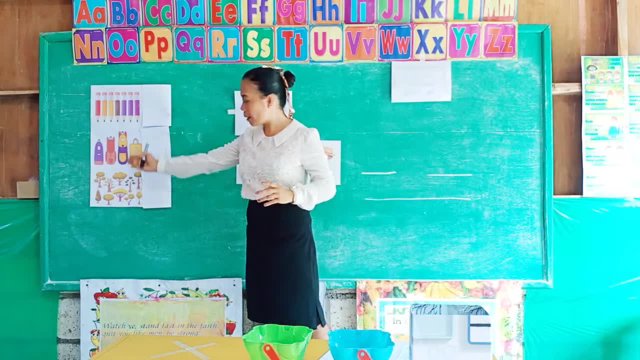 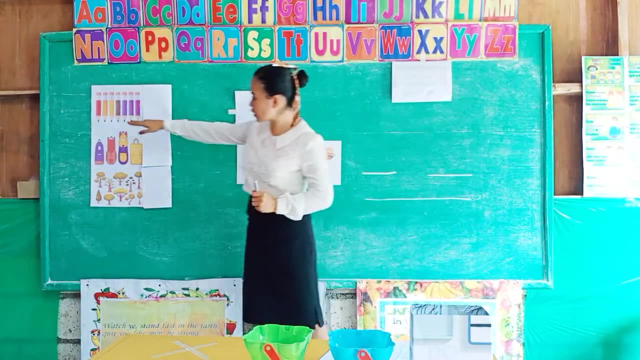 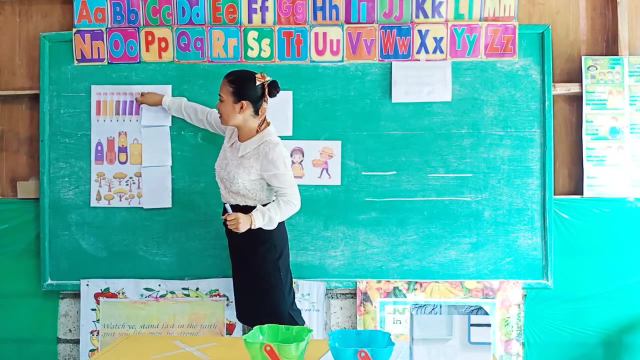 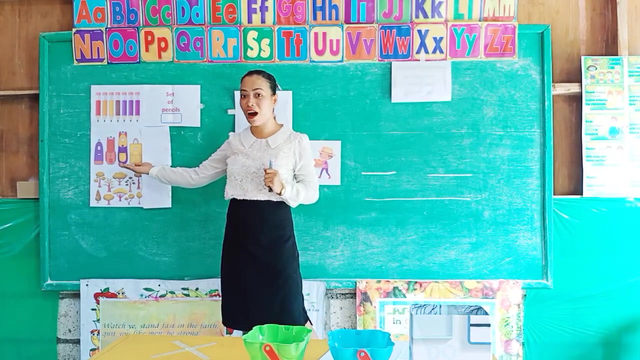 Okay. So please listen, We have here pictures. Can you name these pictures? Okay, Let us name. So, first one, this is a set of correct sets of pencils. Next picture: Very good, This is set of bags. And lastly, we have here: 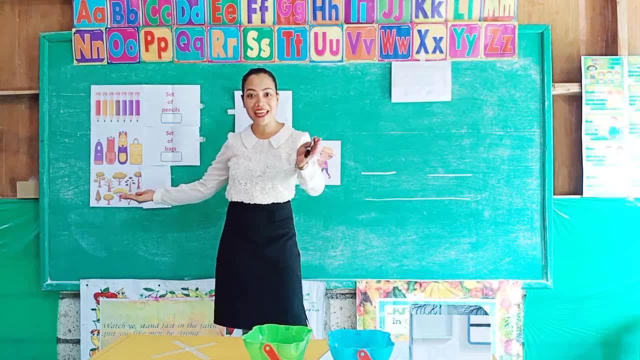 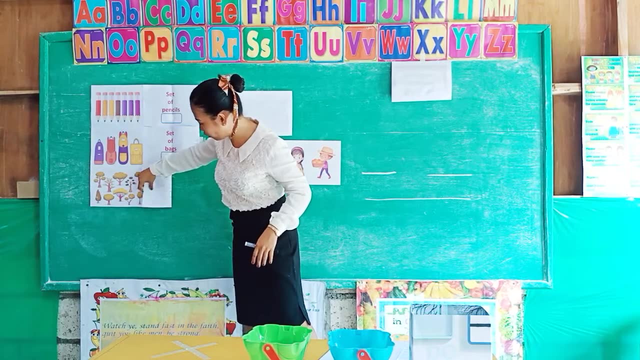 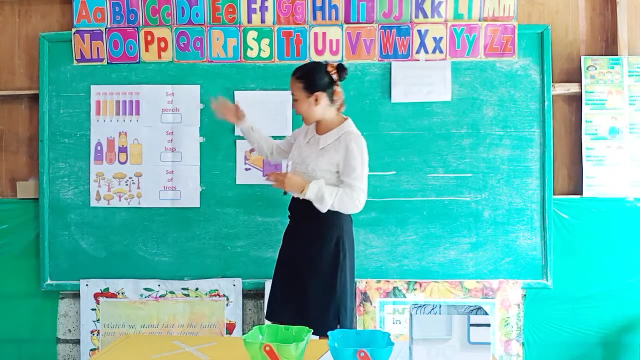 What is this? Okay, Set of trees. Correct grade 1. This time. so you already know what are the sets or the objects. This time. we will count it together, We will count it all. You know how to count. 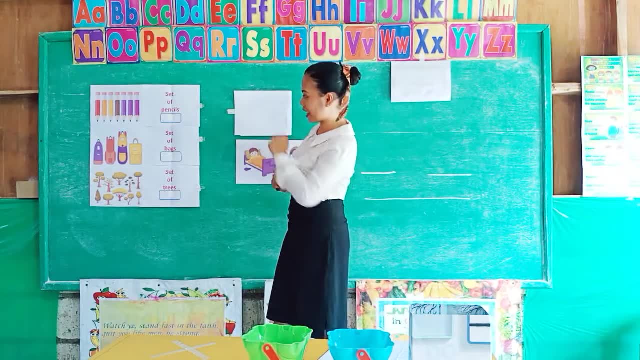 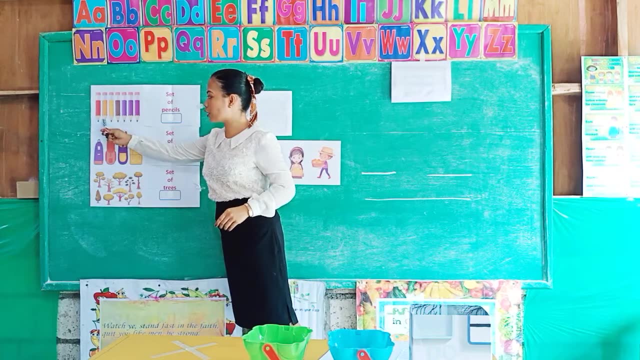 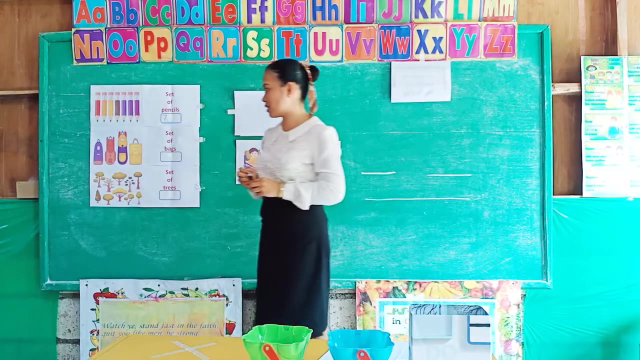 Okay, Let us try to count All the sets. First one is sets of pencils. We will count children. Let us start 1, 2, 3,, 4,, 5,, 6, 7.. So there are 7 pencils. 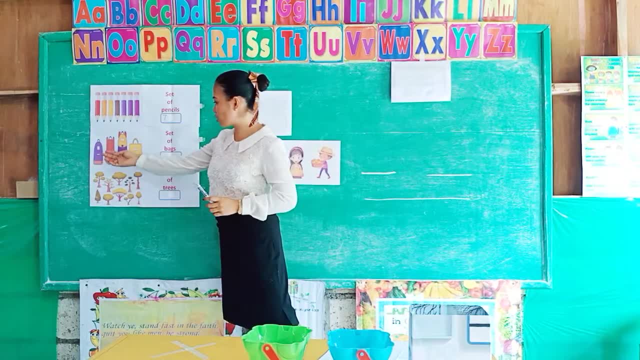 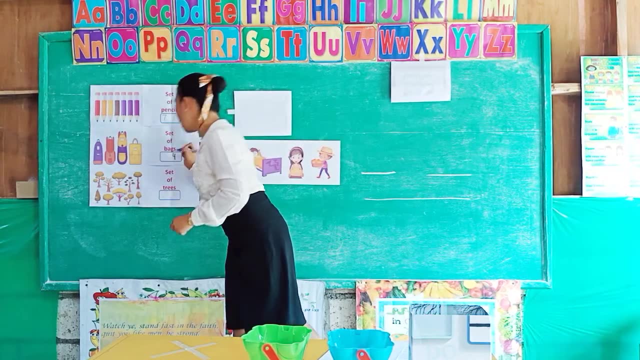 Next, one sets of bags. Let us try to count: Start 1,, 2,, 3,, 4.. So we have here 4 bags And lastly, we have here, Yes, the set of trees Count. 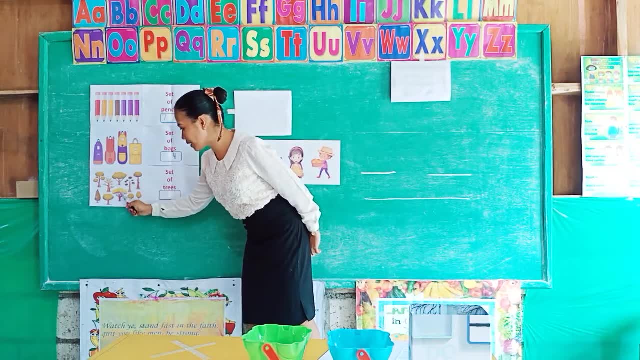 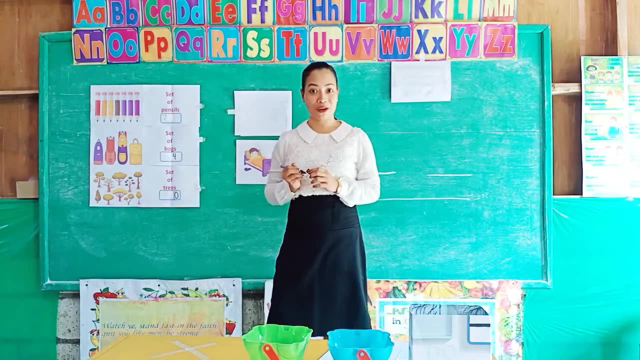 1,, 2,, 3,, 4,, 5,, 6,, 7,, 8,, 9,, 10.. So there are 10 trees. Very good, So now I want you to count the boys. 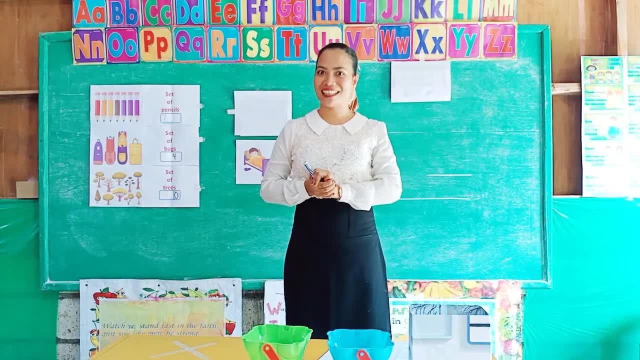 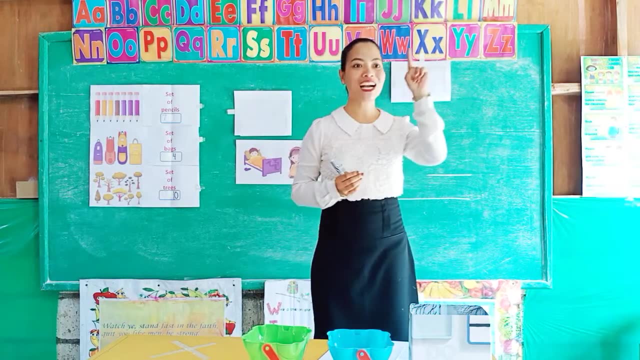 Girls, let's count them all. Let us try to count the boys. Okay, Start: 1,, 2,, 3.. 3,, 4,, 5,, 6.. Very good, So there are 6 boys. 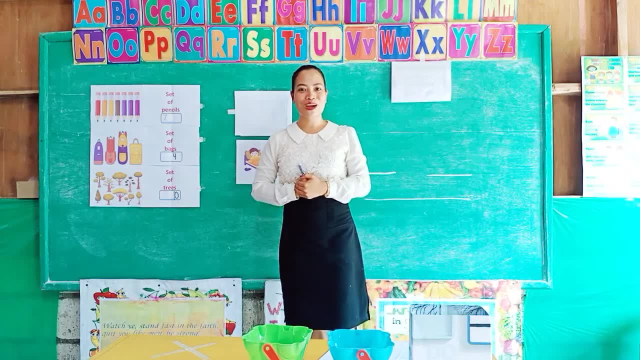 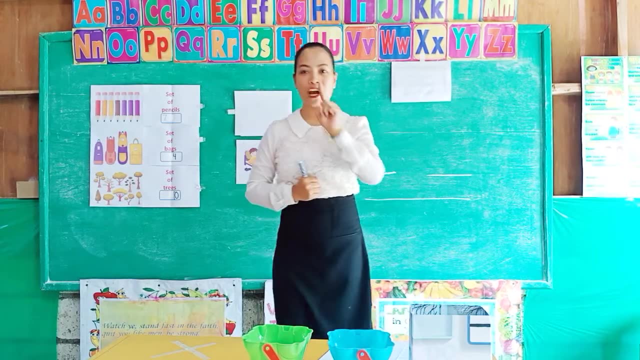 How about the girls? Let us count the girls. Okay, We will count the girls. Let us try to count. Go 1, 2, 3,, 4,, 5, 6.. Wow, There are 6 boys. 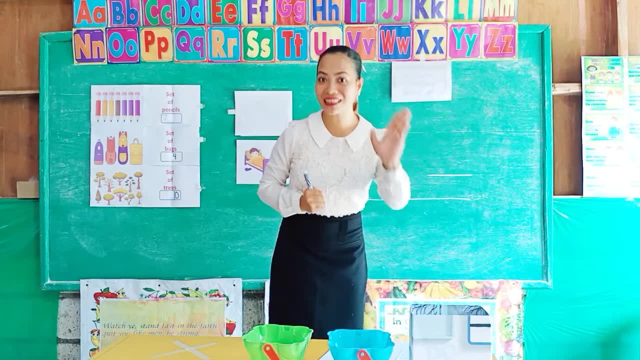 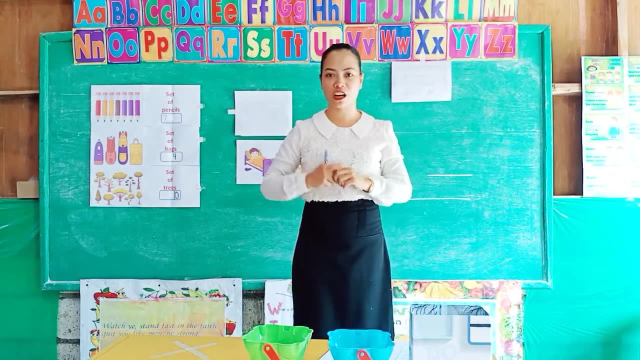 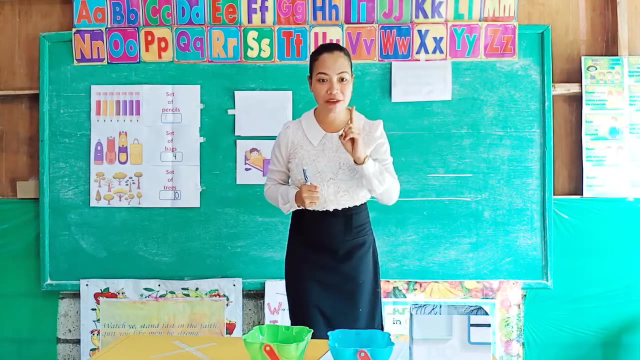 Girls. Let us count them all. All the children are in the classroom: 6 boys and 6 girls. Let us count them all. Go: 1, 2,, 3,, 4,, 5,, 6,, 7,, 8,, 9,, 10,, 11,, 12.. 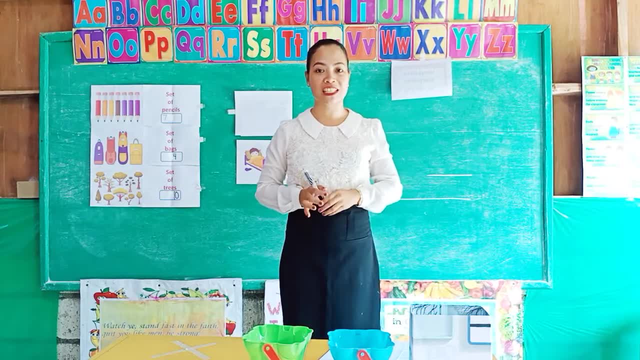 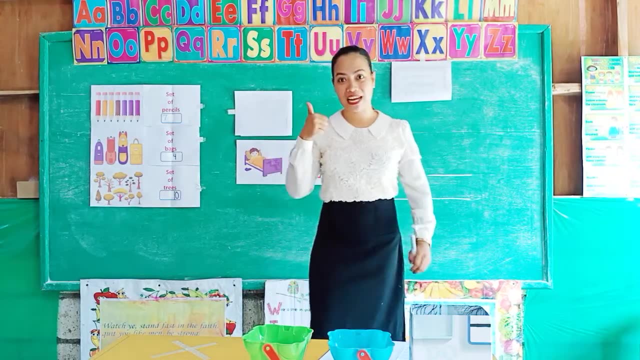 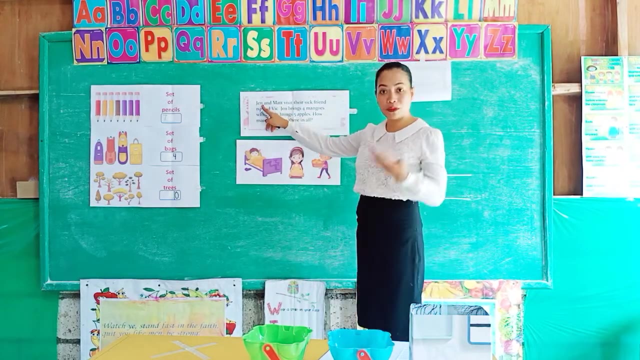 Very good. There are 12 pupils in this class, So is it easy to understand the short story? Okay, So is it easy to understand. I have here a short story I will read. Jen and Matt visit their sick friend named Vic. 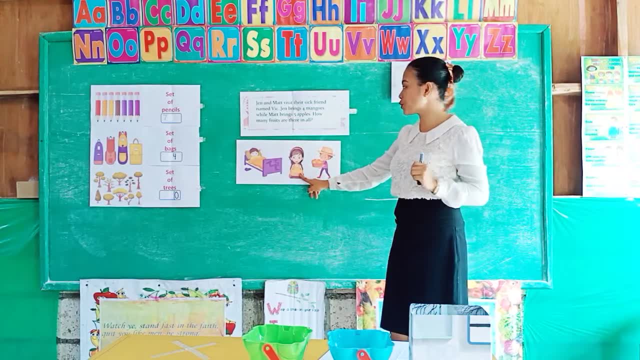 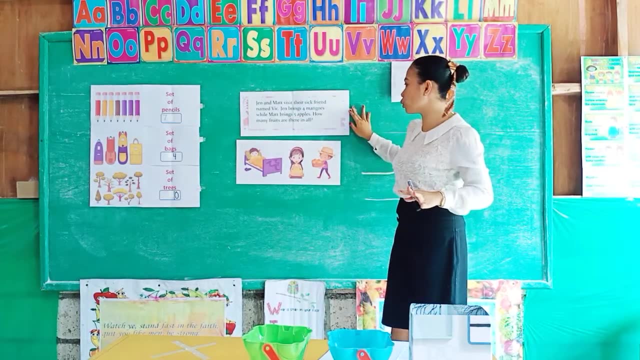 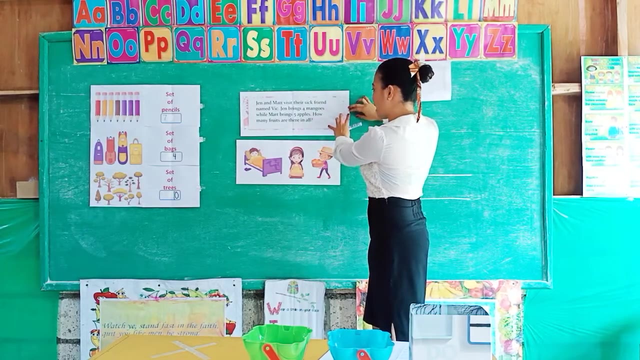 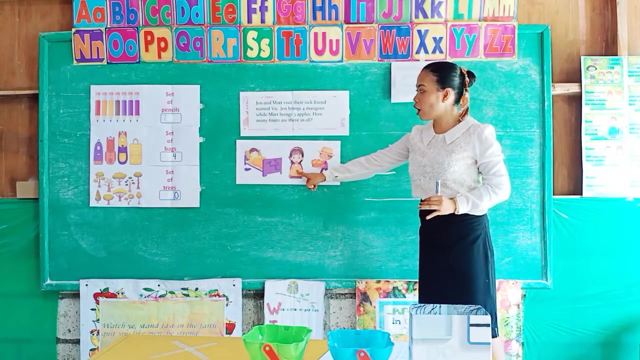 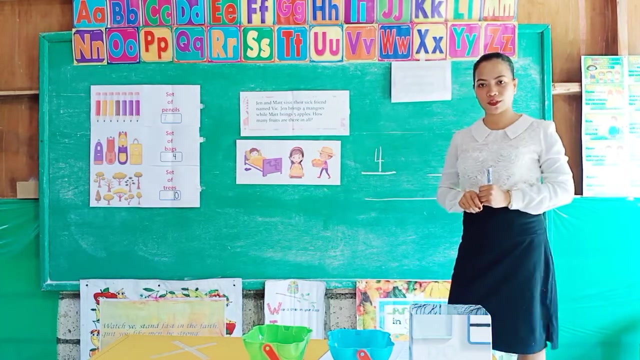 Jen brings 4 mangoes, while Matt brings 5.. How many fruits are there in all? So there are many fruits. There are many fruits for the children and their sick friend. So again for Jen: she brings 4 mangoes, while Matt brings 5 apples. 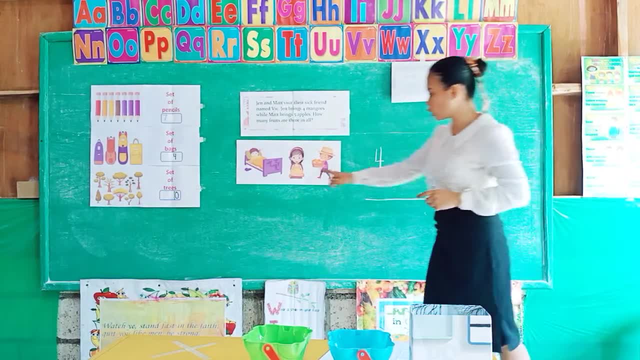 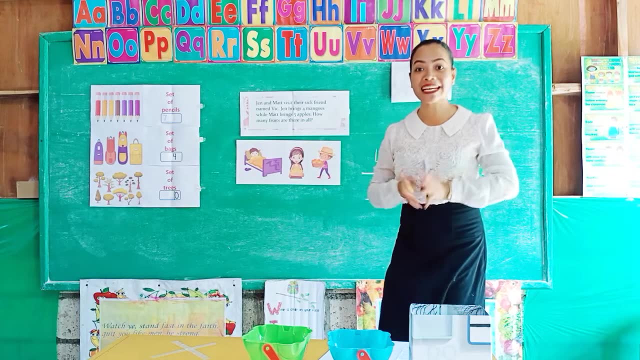 If we will add it together, let us count 1, 2,, 3,, 4,, 5,, 6,, 7,, 8,, 9,, 10,, 11,, 12.. So there are 9 fruits. 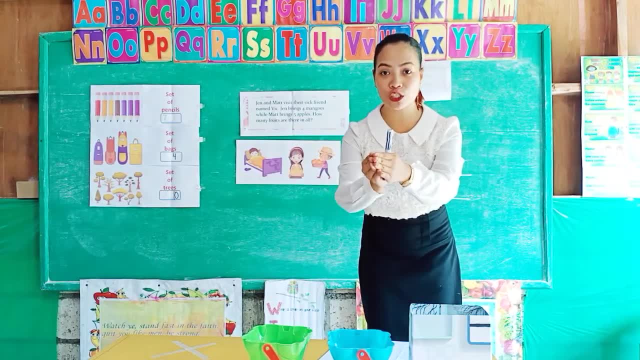 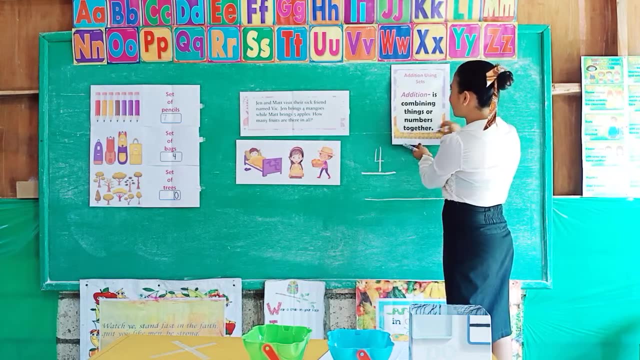 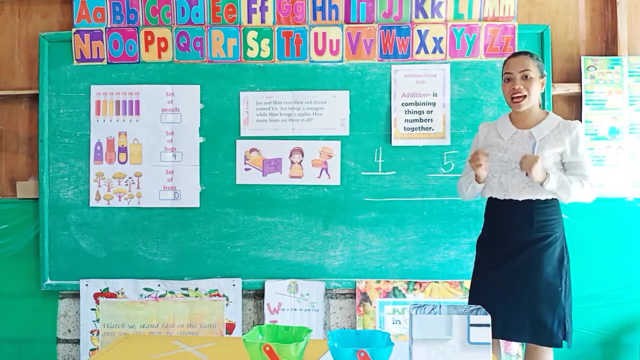 So what is this? Add together, Add together So that process children. Our lesson for today is about addition using sets. Everybody, please say addition using sets. When you say addition, you are adding. Addition is combining things or numbers. 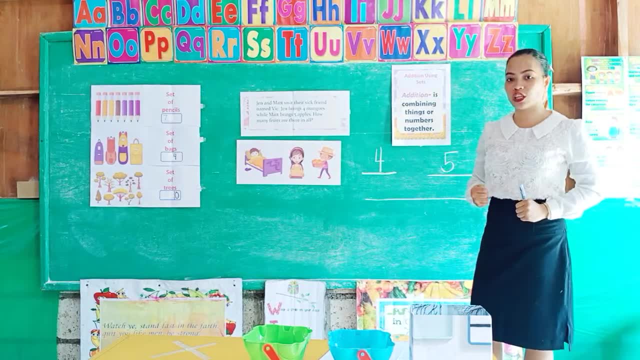 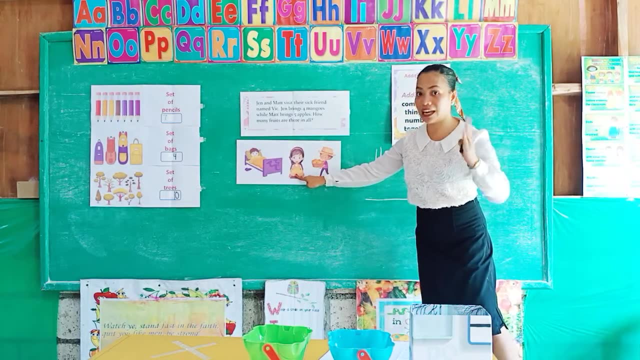 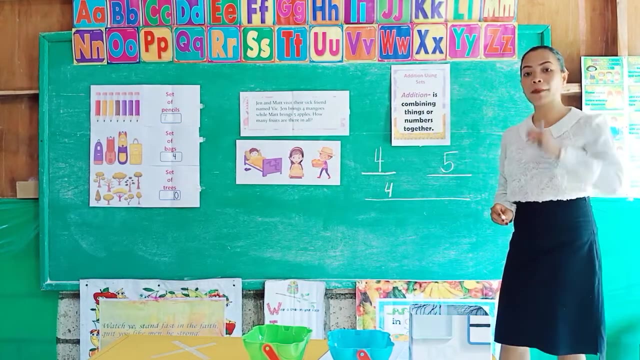 Combining things or numbers together. In adding also children we can write addition sentence. Let us see: First, Jen brings 1 mango. Second, you bring 4 mangoes. How about Matt? He brings 5 mangoes. 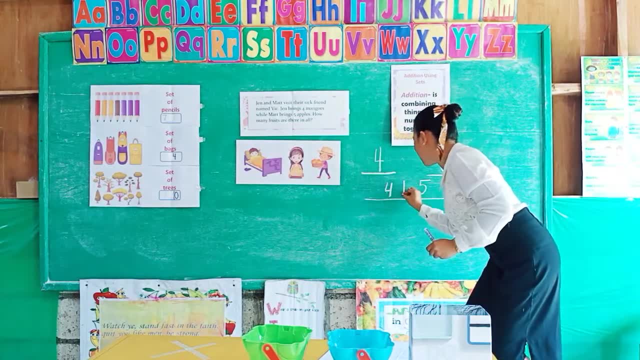 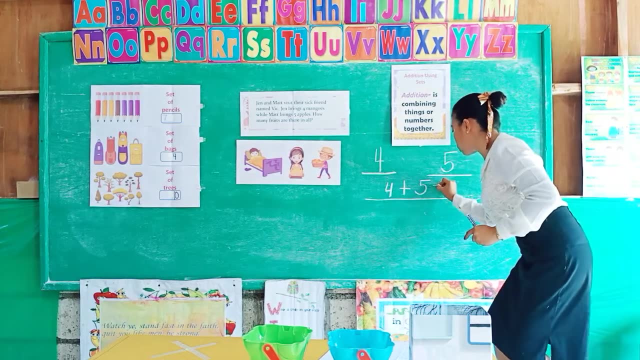 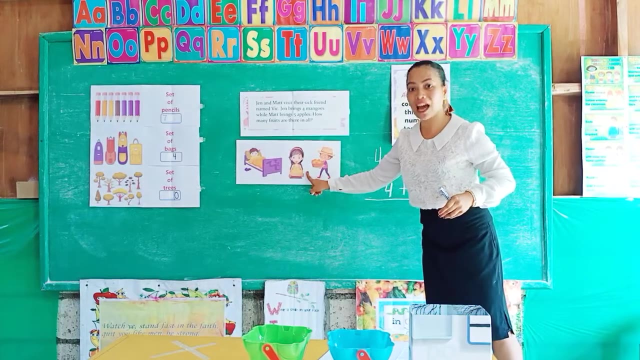 In addition, children, we will use plus sign. Plus sign is similar to T Or yes cross. This one is equal sign If we will put them together. How many fruits are there? Very good, 9 fruits. Did you get it? 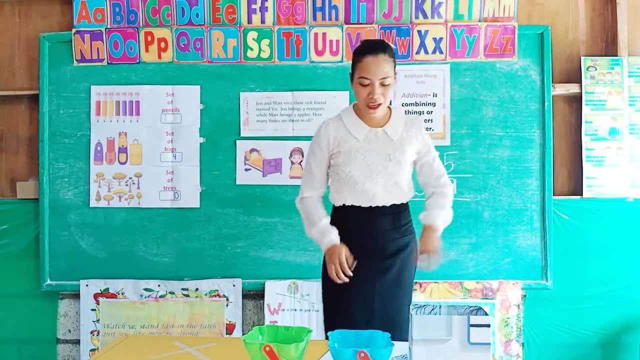 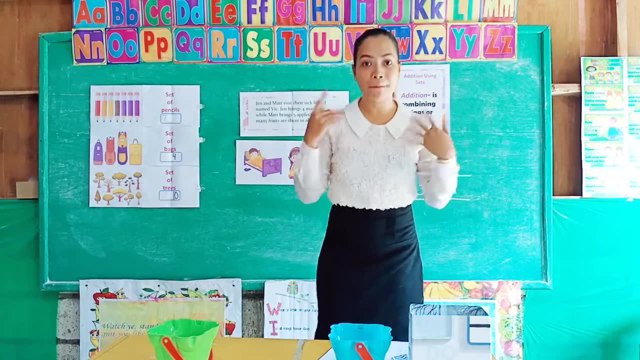 Okay, So we have here, I have here objects. I will add them here. Here is set A, Here is set B: Teacher, you are doing it right If one side is opposite. Teacher, you are doing it right. 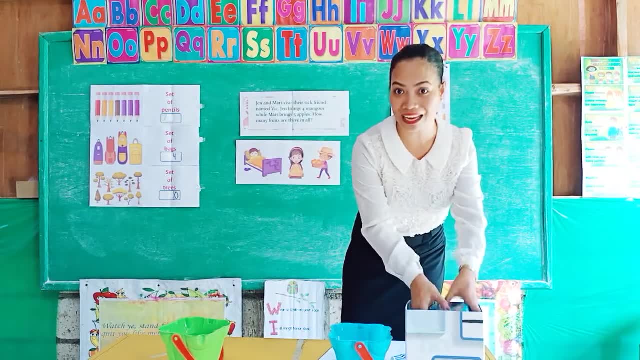 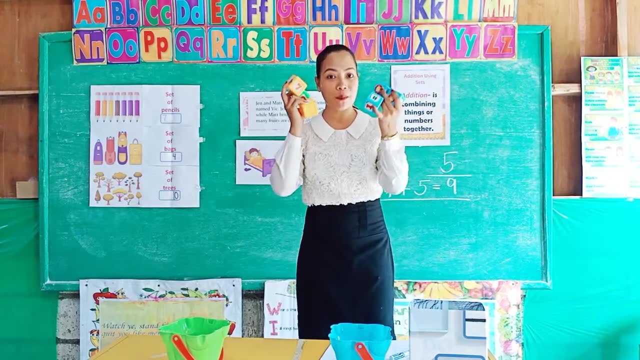 This is set B. I mean set A. Sorry, This is set A. I have blocks here. I have squares, So I have squares here. Let us count 1,, 2,, 3,, 4,, 5, 6.. 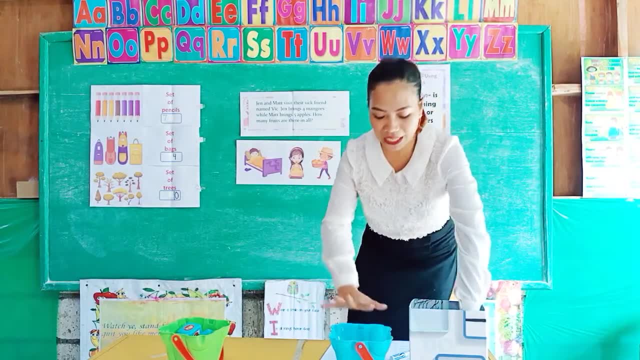 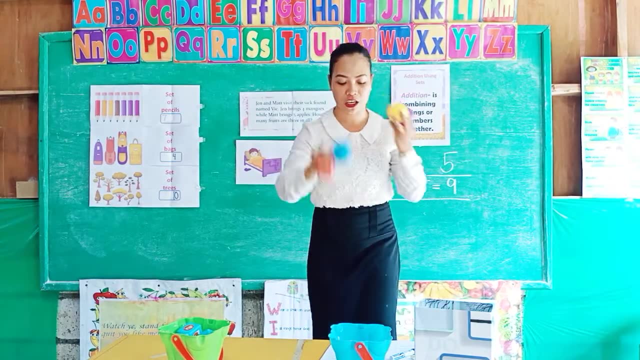 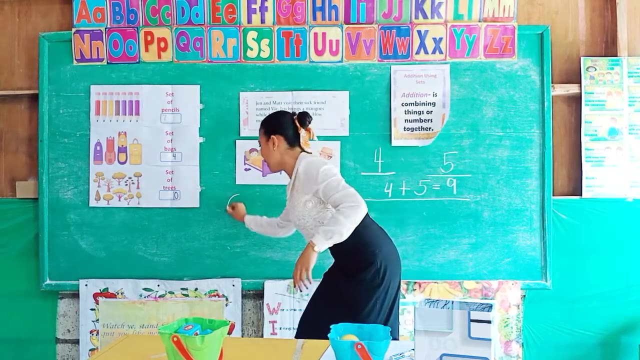 So you have 6 boxes. This is blue basket. children, I have balls here. I have balls here. Teacher, you are doing it right. 1, 2, 3.. One, two, three, four. So now again, dito sa pikas na atay six and dito sa pikas na atay four. 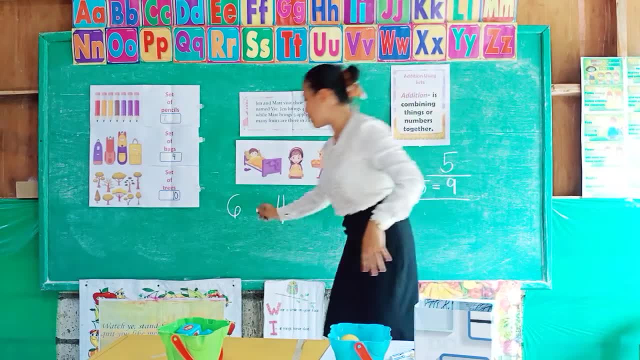 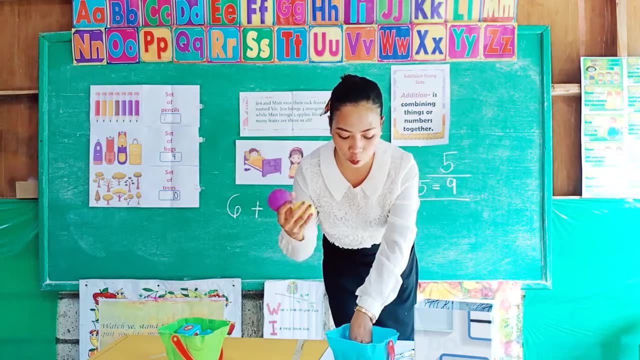 If we will put them together, if we will add pila tanan ka buo, we will use plus and we have here equals: Kung iipo na ito tanan. we have here four and we have here six. 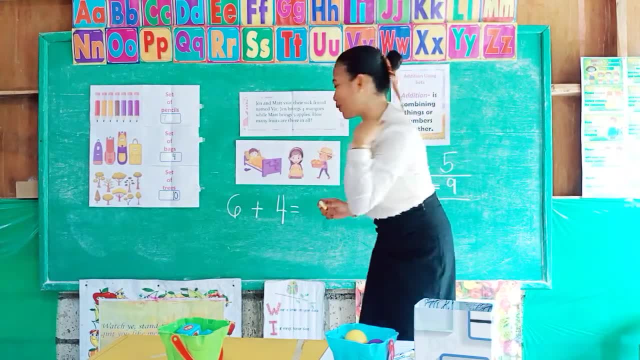 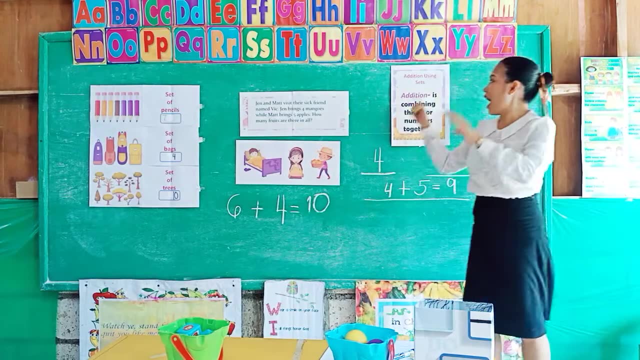 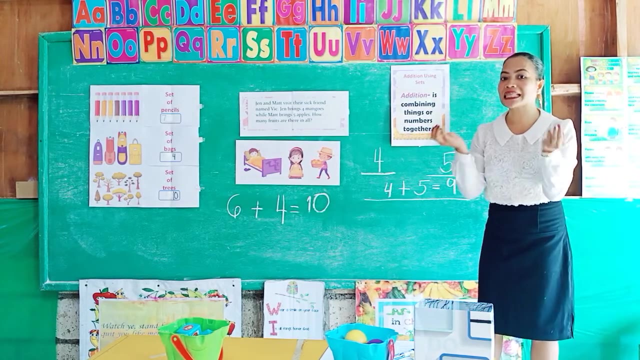 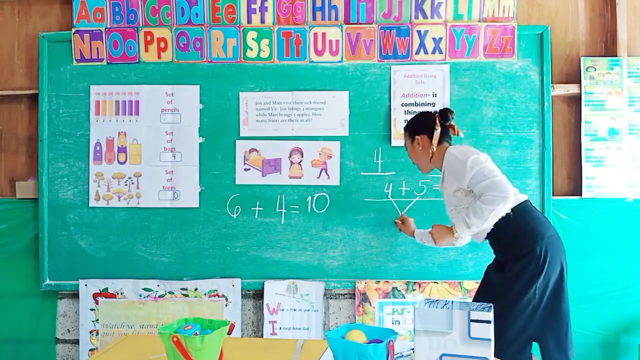 Pila naman tanan In sakto. we have here ten objects, Again, again, children. what is addition? Addition is combining things together. Iipon itapo, And we have here parts of addition. We have here two numbers that we add. 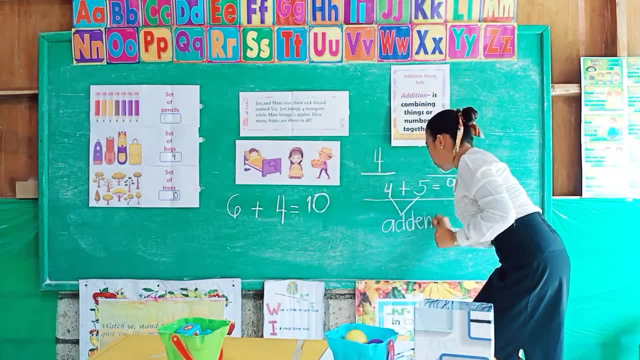 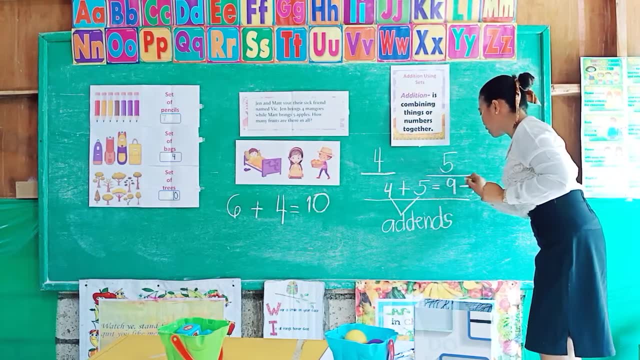 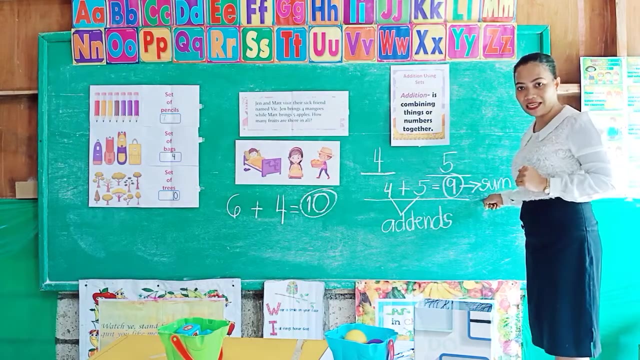 It is called adens. When say tawag again, I can hear you very good, adens. And the answer, this one is the answer, And this is also the answer. We will call it sum Again. kung sa ganito, kung magtaputa, very good. 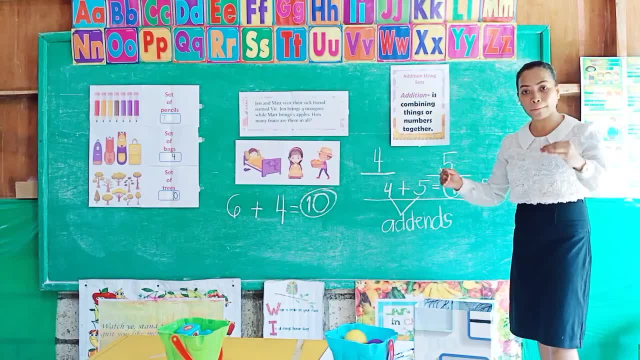 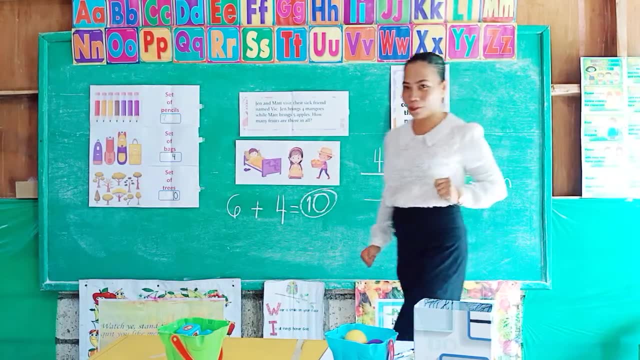 Addition iipon two numbers, or the numbers that we add, is called adens. Very good, and the answer is sum. So now pangunapun ha Kuha ang inyong buta nga naasa inyong bag hindi pa tala nga nung ni teacher no. 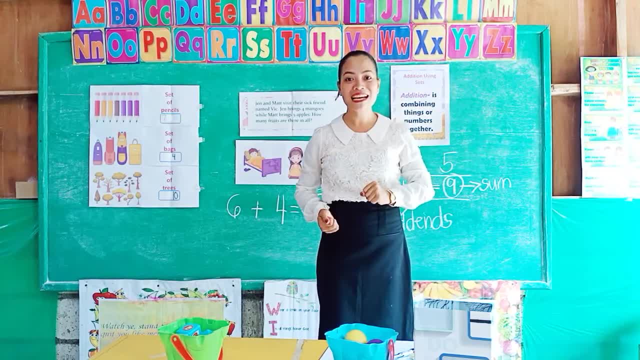 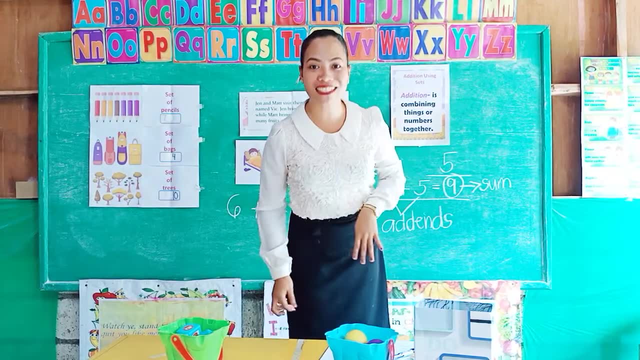 Okay, naapun mo yung box. Okay, ready na. So paminaw ni teacher ibutang sa unang box ninyo four ka-kendis. Oh, nagdabay akong kendis. Go, go, go go. 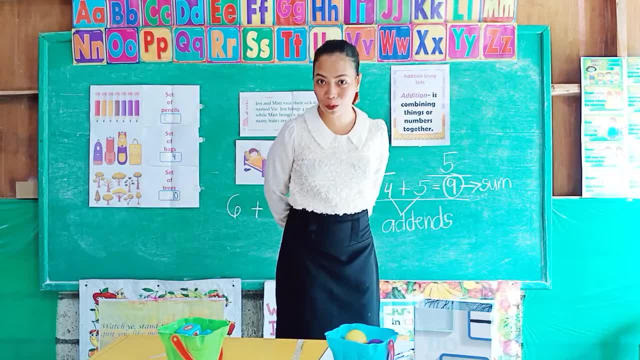 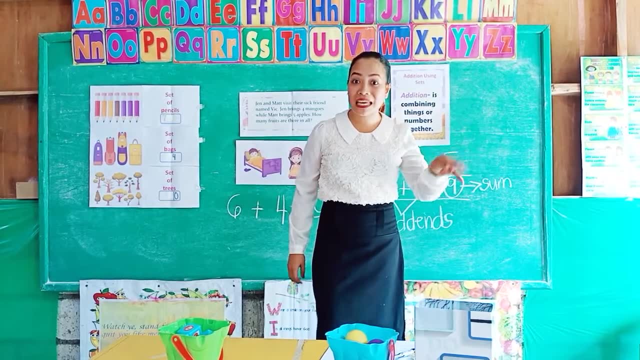 Okay, very good. Now diha sa usang ka-box na punin nyo butangi og tulo ka-kendis. Okay, very good, So naan na Upat sa pikas og tulo sa pikas. 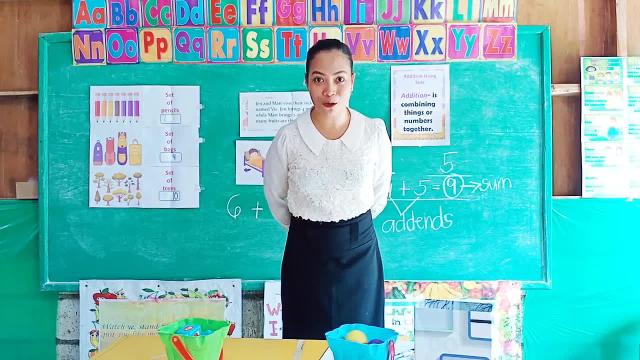 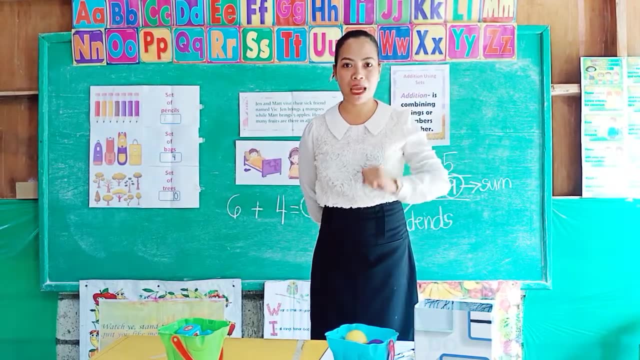 Ipon na tutanan. Very good, you have there seven, Seven. So now, children, I want you to Write the addition sentence in your paper. okay, So write. Then may I see Ay, very good. 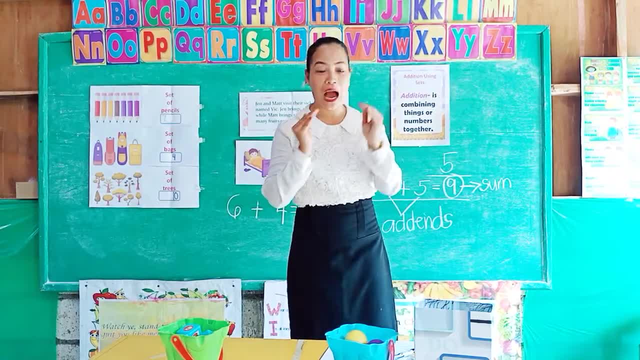 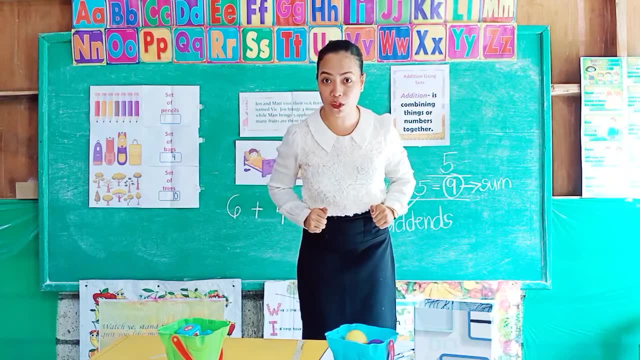 Nasabta na GDI. So that is all about addition. So nasabta na Okay. so karoon ka muna mo answer sa inyong books. okay, Please get your book and open it. on page 85, and please answer it. 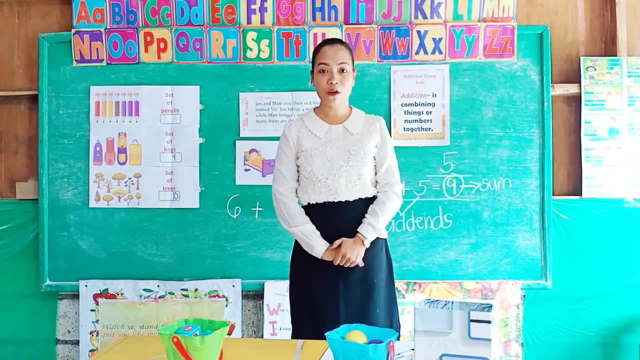 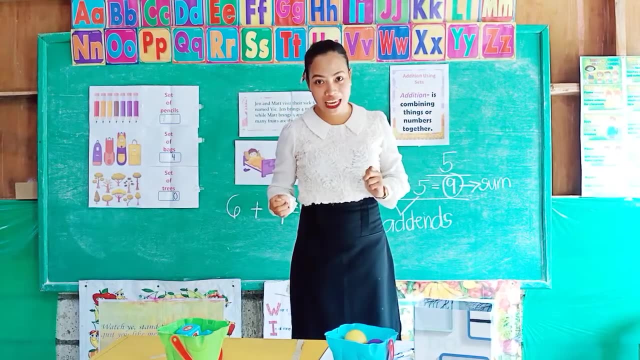 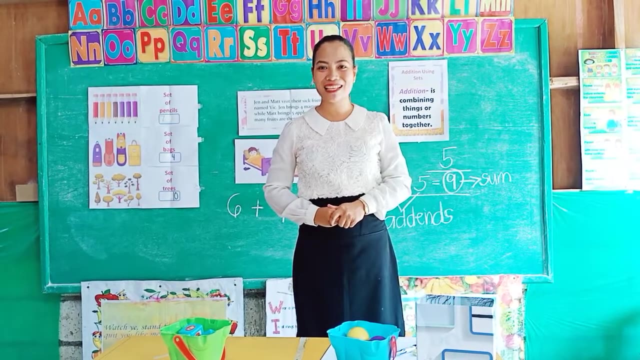 Go Very good. So now please keep your book and children for your assignment. please study the properties of addition. okay, That's it for today. Goodbye, and God bless you.